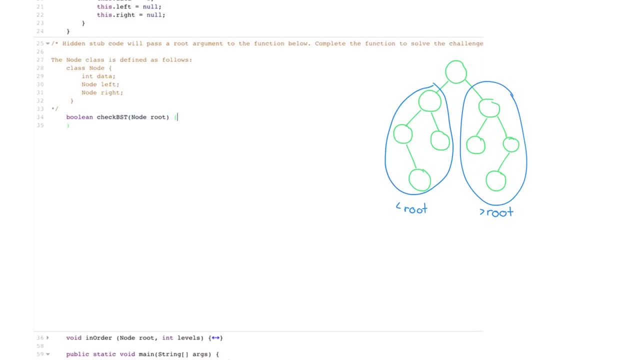 nodes on the left for any given node, all the nodes on its left are smaller than it and all the nodes on its right are bigger than it. So we want to check to make sure a binary tree is actually a binary search tree, and so that means checking to make sure that ordering property is. 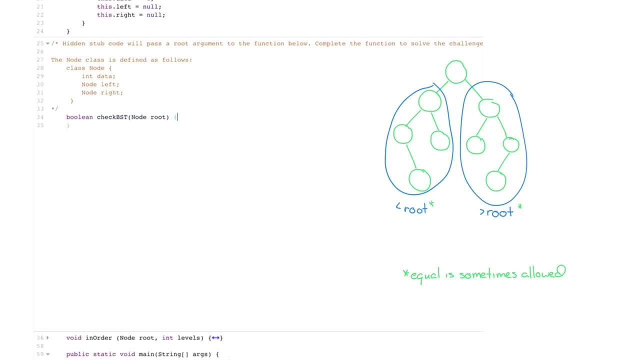 true. So one approach that a lot of people take that is actually mistaken is they think: okay, I'll just walk through my tree and check to make sure for any given node, compare it to the left node, compare it to the right node and see if it's in the right order. So is the left node. 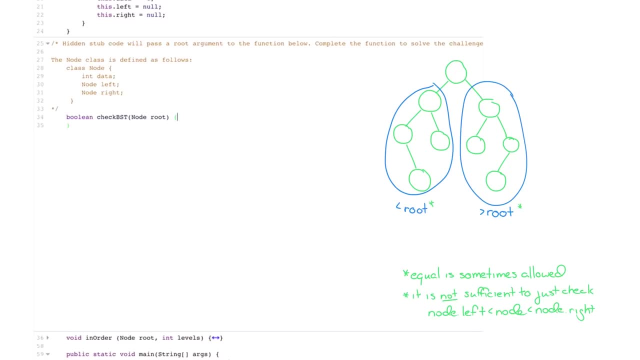 smaller than the current node and smaller than the right, And the problem with that is that, even if that's true, it may not be a valid binary search tree, because there could be something, something else underneath it that's bigger than the parent. So for any given root, 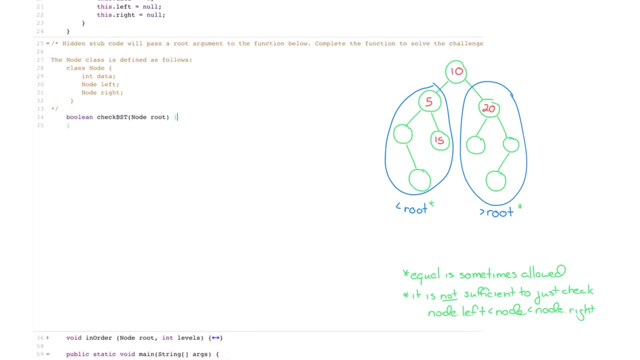 maybe it's grandchild is actually bigger than it, and maybe it's left grandchild is actually bigger than it. So that won't actually work. Another approach that is correct but slow is we can say: okay, all the nodes on the left must be smaller than all the nodes on the right, So take. 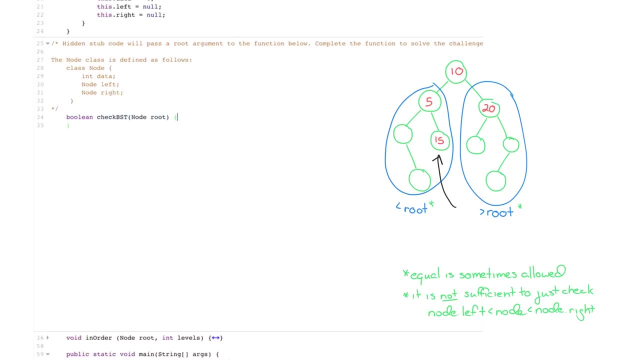 each node. get the biggest node on the left, compare it to this node. get the smallest node on the right, compare it to that node. That'll work, but it's pretty inefficient. These get min and get max operations require walking through that whole tree. So we want to check to make sure that all 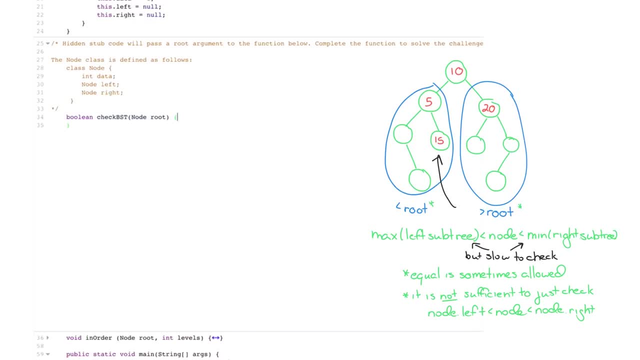 the nodes on the left are min and max. operations require walking through that whole tree, So that's going to actually get very, very slow. A faster way is we can flip around this logic. We can say, okay, at the very beginning, our root is valid. The root can be anything in the entire world, But 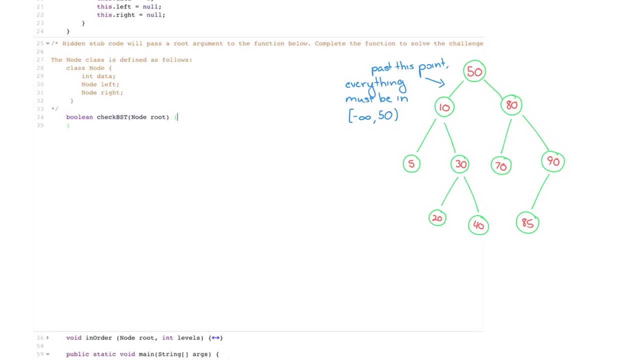 when we go to the left, we're going to walk through all of its children and we'll go to the left. everything on the left has to be between the integer minimum and the root value, And everything on the right has to be between the root value and integer maximum. 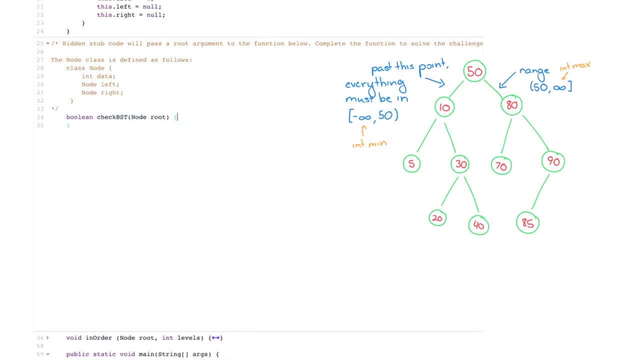 So take the chez function. Please go to the left. Well, we'll check to make sure. Hey, is that node on the left? Is that within those values? Great, it is Okay, keep going. Now we want to go to the right side of that. All those values must. 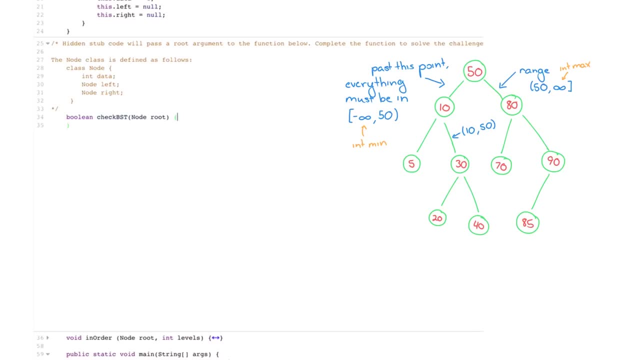 be between that left node's value and that root node's value. So we're going to pass around these ranges of min and max And say at every any given point: Okay, is that min? Yeah, That's all it makes. 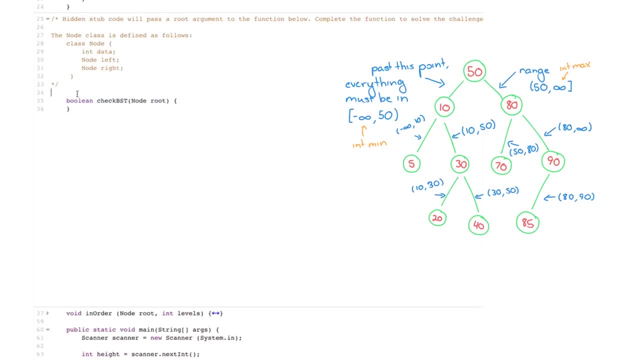 range. So that's how we tackle this problem. Okay, so we need for this method actually is: we need checkBST to take in a min and max value, And this initial node is going to just take in a passInIntegermin. So initially, the root. 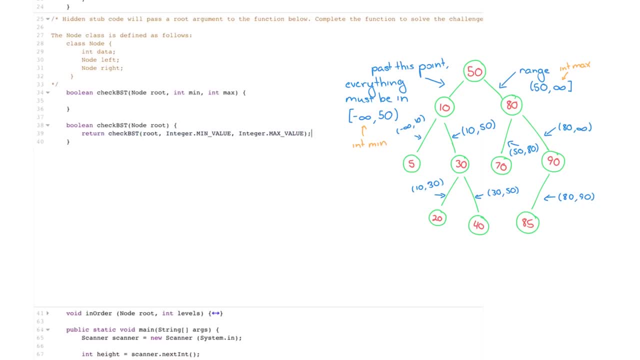 can be any value at all at all. actually, Now I'm gonna make sure I'm gonna specify here: these are inclusive ranges, Okay, so in the very beginning, first I want to do so, I want to check to make sure my root is in the right value. So if it's smaller than my min. 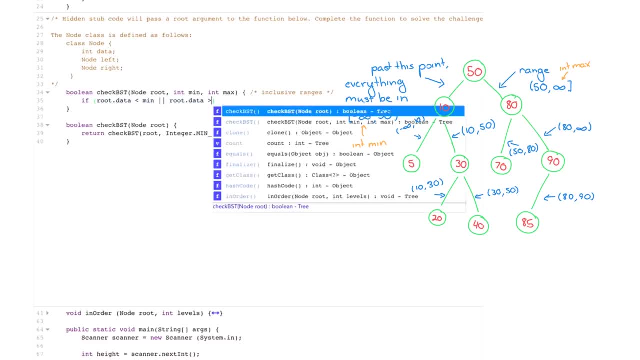 or it's bigger than my max, return false. I also want to be careful of I need a base case here. so if root is null, then return true, otherwise go left or right. so check my left and right root: dot, dot left, and I'm going to come back to what. 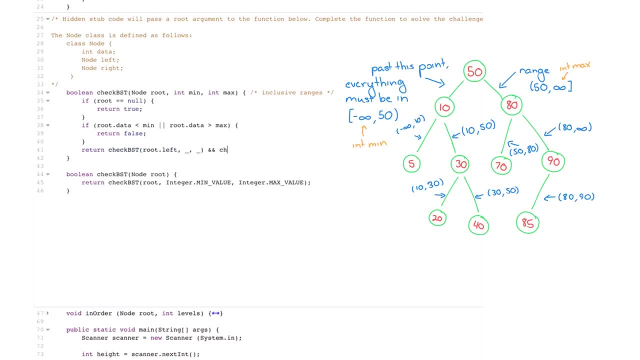 these ranges are in a second. so check the left and check the right. if both are valid, then it's valid. okay, that's a basic logic. now, initially my, so my root can be in between min and max if I go to the left of my root, anything down there. 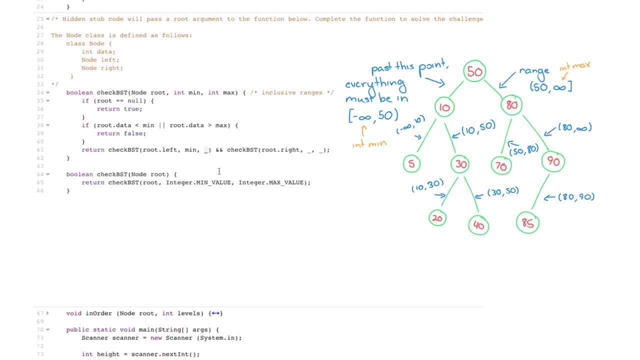 can still be as small as the min, but it cannot be any bigger than the, than the root, and in fact it can't even be equal to the root because we actually do not have duplicates in this tree, and so the biggest. so my values on the left of my root can be anywhere between min at the. 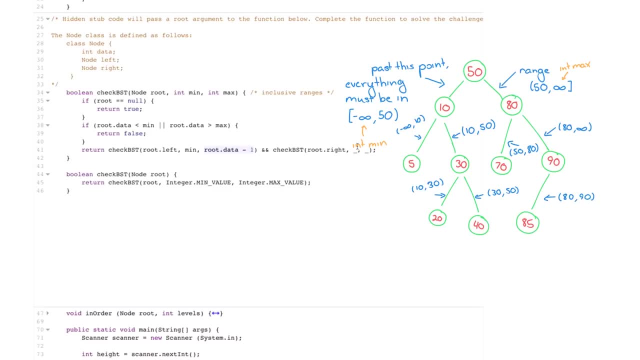 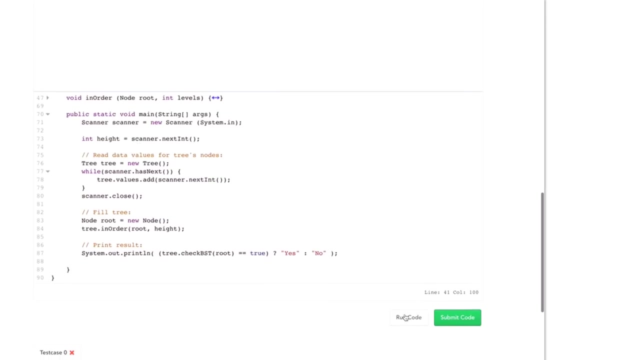 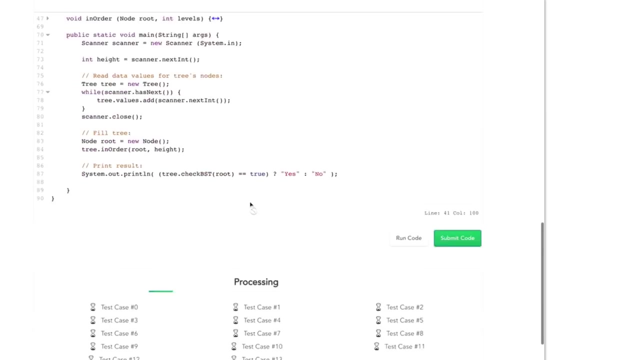 smallest and one smaller than the root. when I go to the right things can be at least- or they have to be at least as big as root, actually one bigger and they can be up to that max value. now let's run this and see what happens. perfect, it worked. so we can do it so in more test cases if